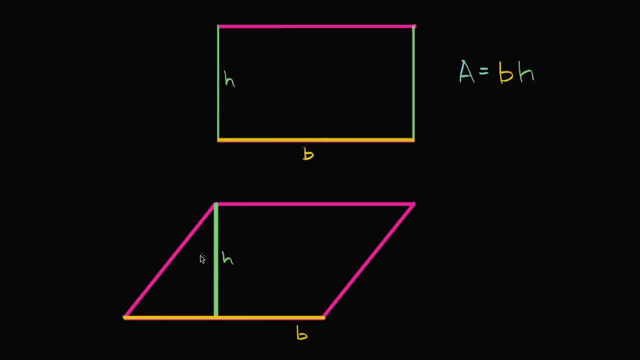 You just multiply the base times the height. Now let's look at a parallelogram, And in this parallelogram our base still has length b and we still have a height h. So when we talk about the height, we're not talking about the length of these sides. 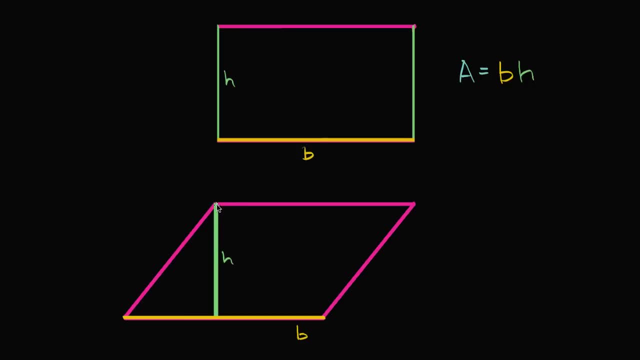 at least the way I've drawn them- move diagonally. We're talking about if you go from this side up here and you were to go straight down, if you were to go at a 90 degree angle, if you were to go perpendicularly straight down. 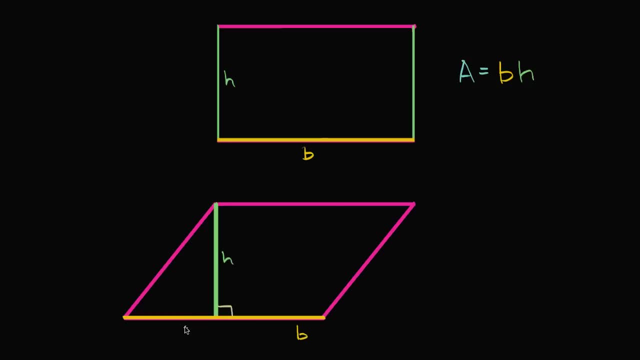 you get to this side, that's going to be our height. So in a situation like this, when you have a parallelogram, you know its base and its height. what do we think its area is going to be? So at first it might seem well, you know. 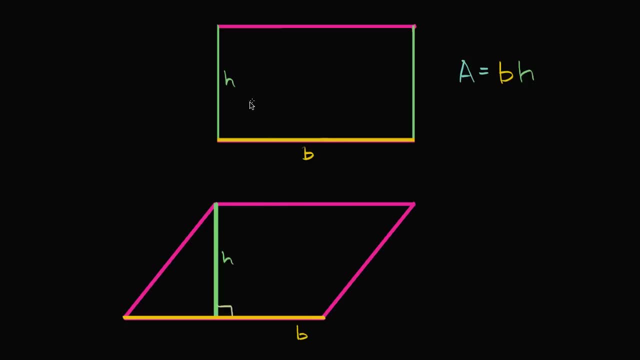 this isn't as obvious as if we're dealing with a rectangle, but we can do a little visualization that, I think will help. So what I'm going to do is I'm going to take a chunk of area from the left-hand side, actually this triangle on the left-hand side. 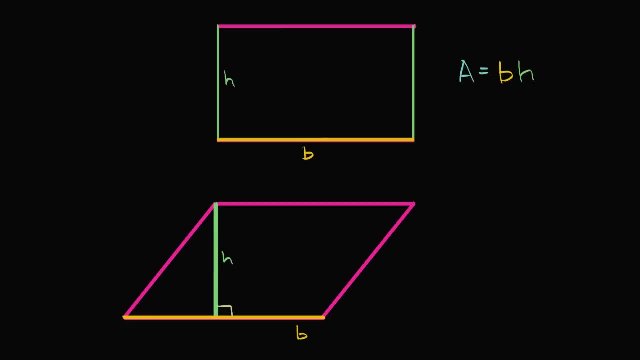 that helps make up the parallelogram, and then move it to the right, And then we will see something somewhat amazing. So I'm going to take this, I'm going to take this little chunk right there. Actually, let me copy it. 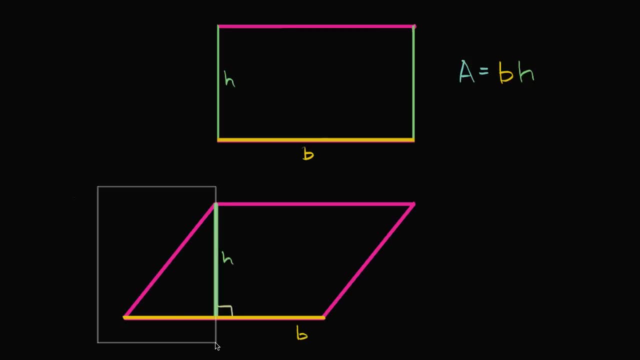 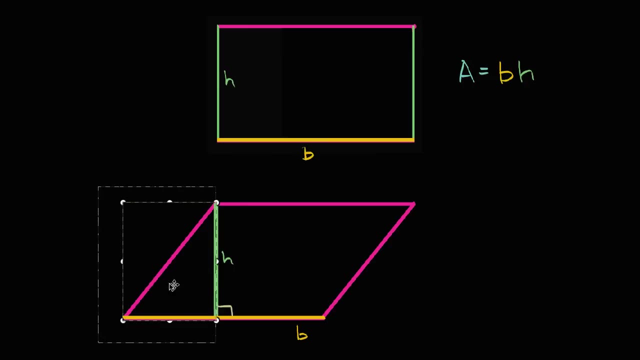 Let me do it a little bit better. So this: I'm going to take that chunk right there and let me cut and paste it. So it's still the same parallelogram, but I'm just going to move this section of area. 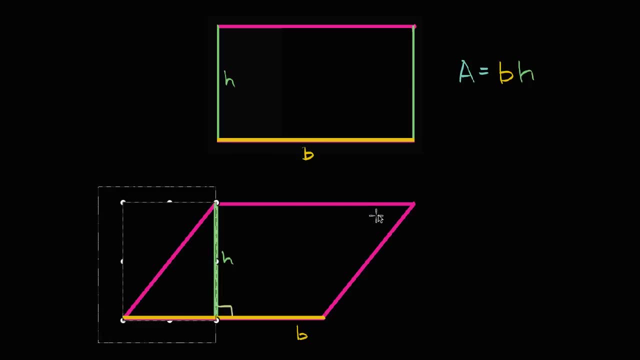 Remember, we're just thinking about how much is space is inside of the parallelogram, and I'm going to take this area right over here and I'm going to move it to the right-hand side. And what just happened? what just happened, 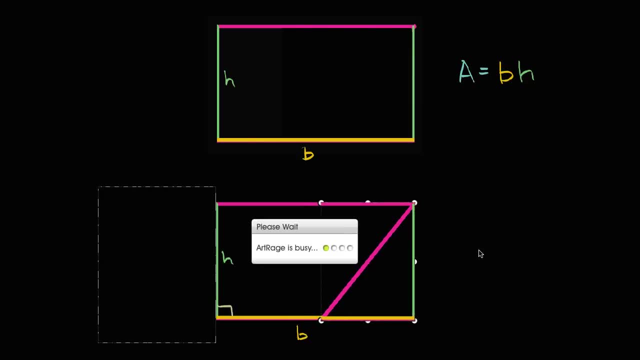 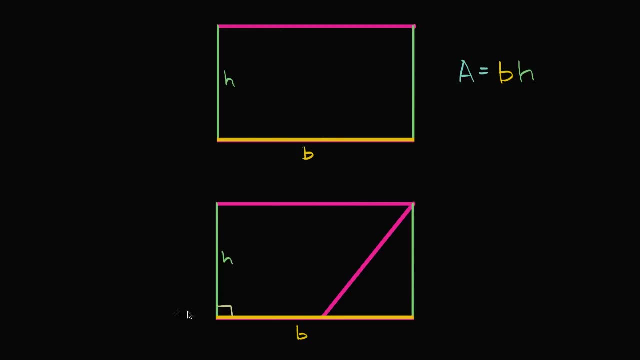 let me see if I can move it a little bit better. What just happened when I did that? Well notice it now looks just like my previous rectangle, That just by taking some of the area, by taking some of the area on the left. 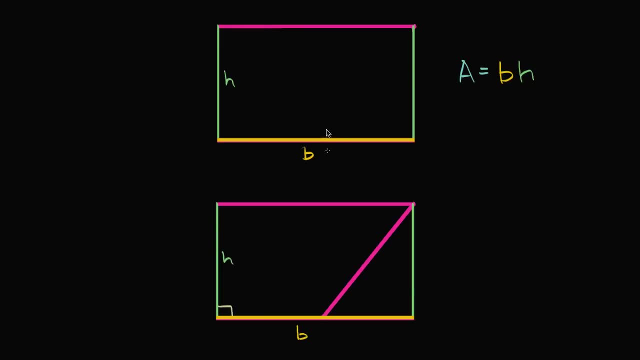 and moving it to the right. I have reconstructed this rectangle So they actually have the same area, The area of this parallelogram, or what used to be the parallelogram before I moved that triangle from the left to the right.